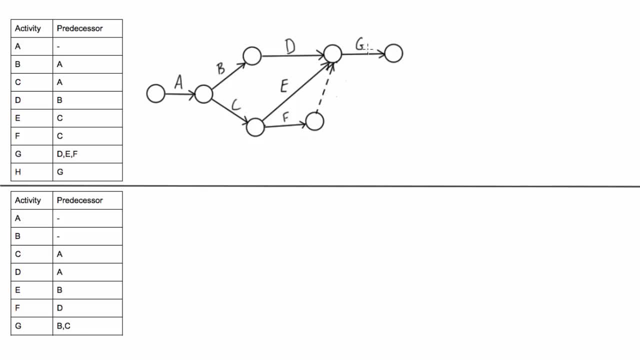 one dummy activity and we still have all of the coração predecessors for G right. So D leads into this point where G can start. E leads into this point and then F, by extension of this dummy, it leads into this point, So F needs to also be done. 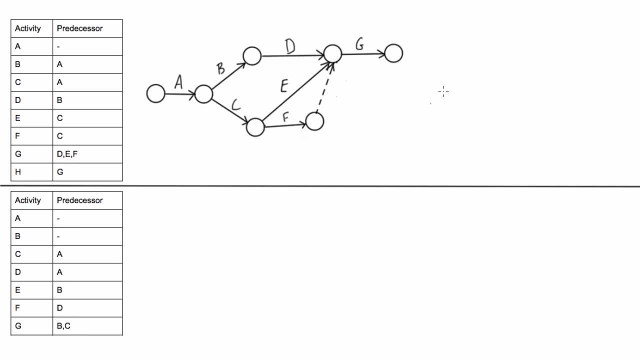 before G can start. So next we've to do is just draw in activity H, And then the last thing we need to do is we need to number each node in a way that every arrow points from a lower number to a higher number. So I would do it this way. This way, we can use these numbers as what's called a unique. 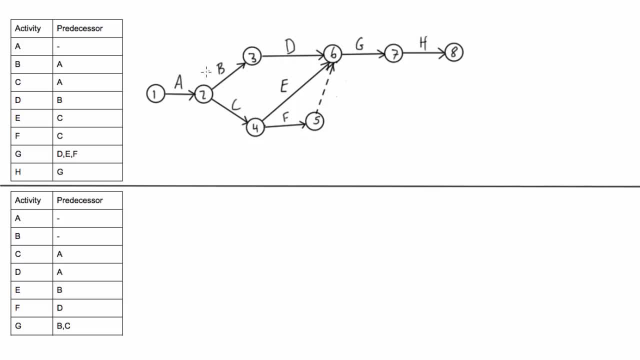 IJ number to identify activities as an alternative to using their name. For example, A's IJ number would be 1, 2.. B's IJ number would be 2,, 3.. E would be 4,, 6. And if you notice every single. 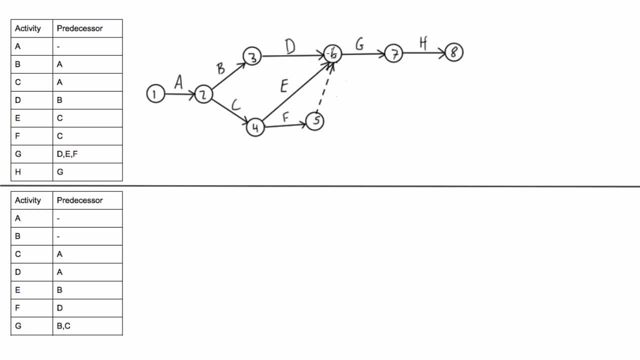 arrow is always pointing from a lower number to a higher number, And if that's correct, or if that's the case, then you know you've done it correctly. All right, so let's move on to the next example here, because this one is done. For the next example we have: activities A and B are: 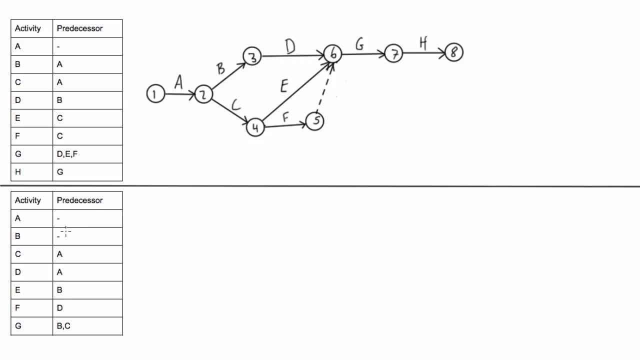 both at the very beginning of the project, because they have no predecessor. But one of the limitations of the CPM network diagram is that you can only start on one node and you can only end on one node. So first of all we'll have to draw a single node with arrows coming off for both activities. A. 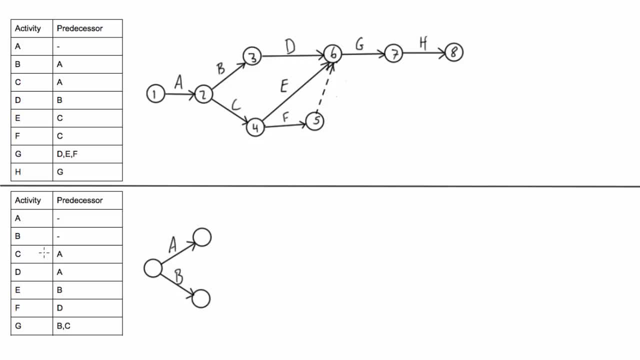 and B. All right. so next up we have activities C and D. Both depend on A, so we can have an arrow coming off for C and an arrow coming off for D. Then next up, we have activities C and D. Both depend on A, so we can have an arrow coming off for C and an arrow coming off for D. 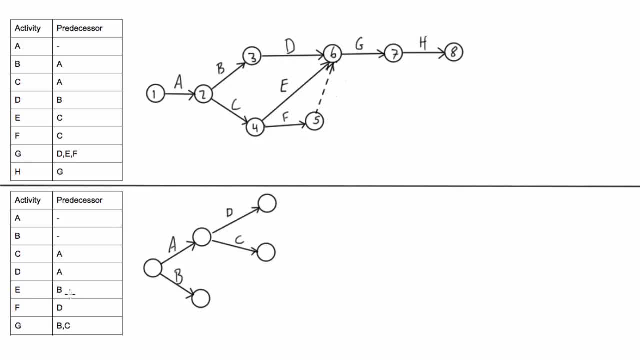 Next up, we have activity E. It depends on B, So let's go ahead and draw an arrow coming off of B. Then we have activity F. It depends on D, So let's just, let's try this out. Let's just draw another. 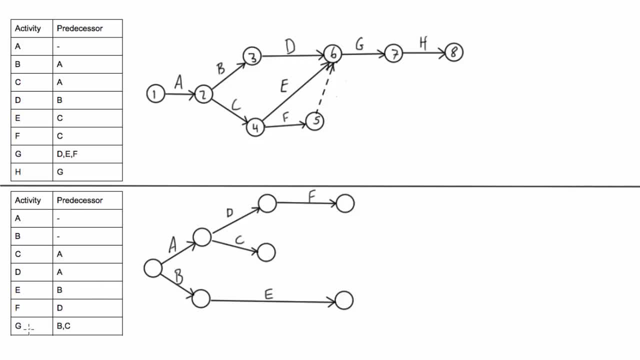 arrow coming off of D. And then, lastly, we would have an activity G and its predecessors are B and C. So we're going to need to come off of C and then connect B to this node with the dummy, But this is going to leave us with three nodes at the end of our project. If we wanted, we could. 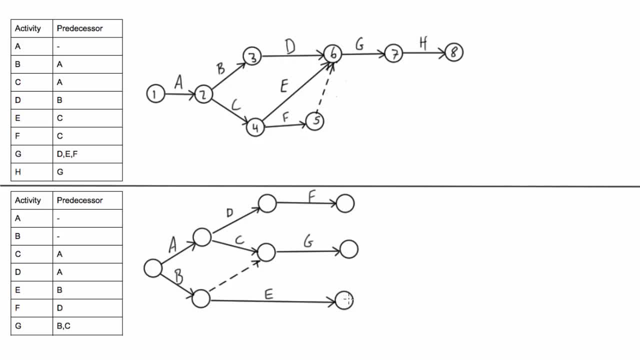 draw on dummy variables. but we're not going to be able to do that. So we're going to have to draw on dummy variables connecting F to G and E to G or to this node at the end of G. But then we're just.